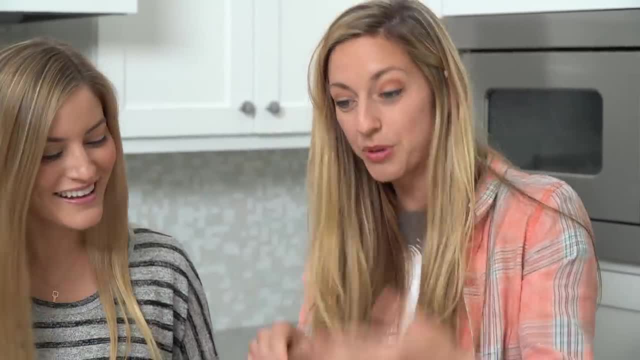 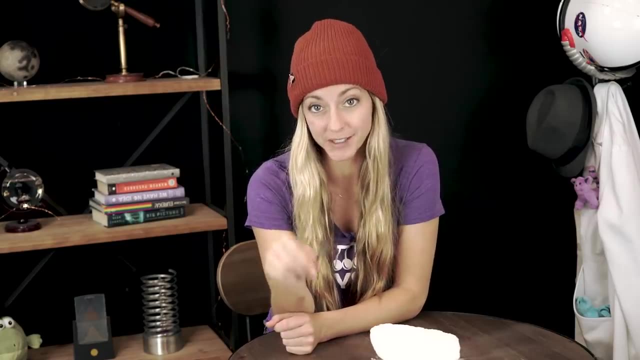 But then you're pressing it down so it goes back on to the dry ice And then it'll push it away and back and forth And that sort of vibrating back and forth will make it scream. This only works with thermally conductive materials. 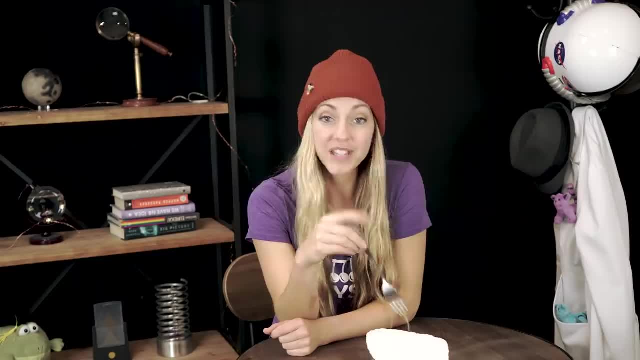 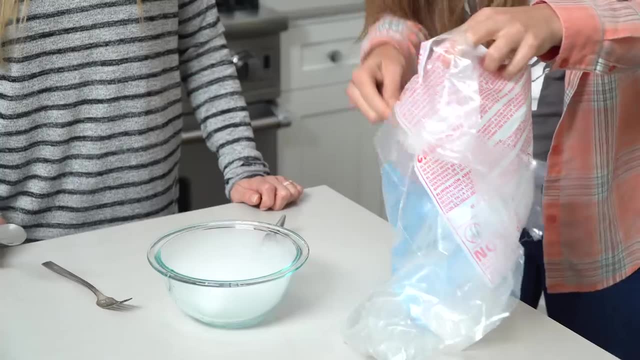 like metal. Feel it. Feel the metal now. Yeah, it's freezing. It feels really cold. These materials, like metal, heat up the dry ice very quickly but in turn become very, very cold. I was trying not to do this when I was starting. 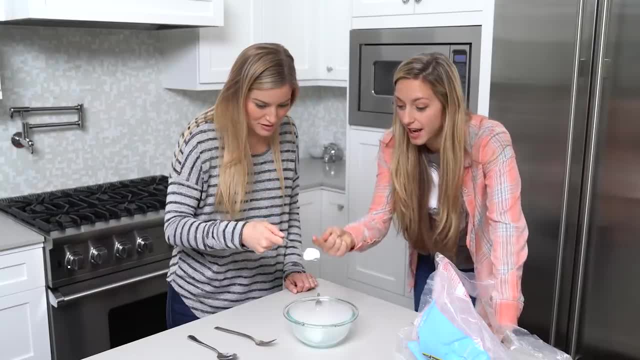 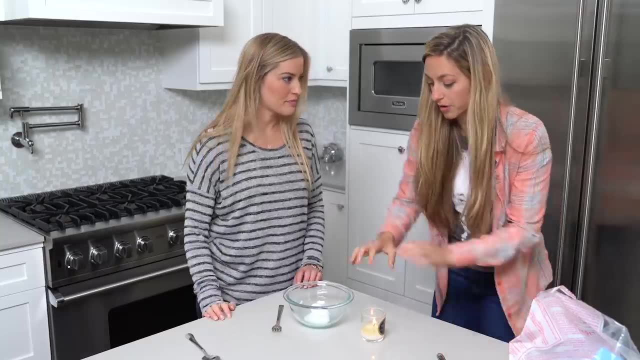 You can see it vibrating. No way, Yeah. And you can also see that carbon dioxide. like: which way is it going? Yeah, it looks like it's going down Down. yeah, Since the gas is more dense than the air. 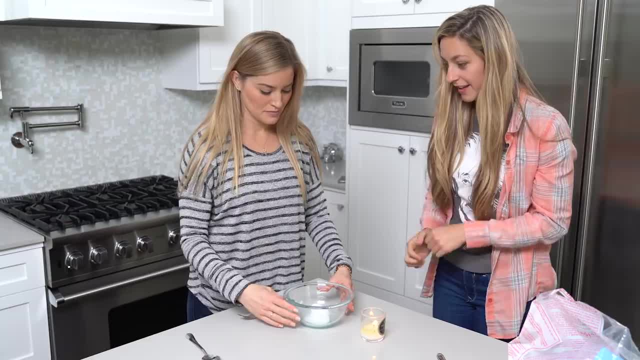 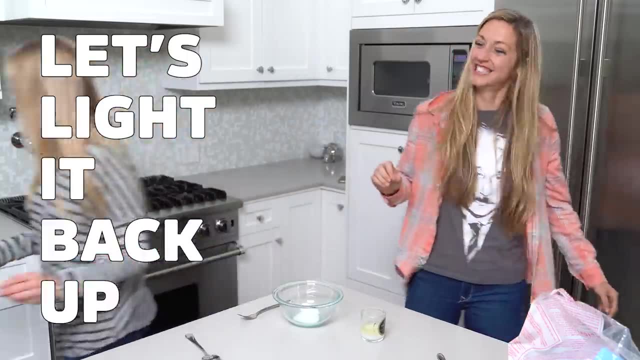 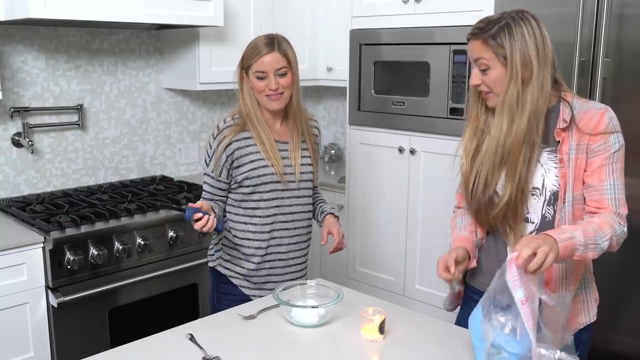 if you carefully pick up the bowl, you can pour that into the candle. No way, That would be so cool. Let's light it back up. This is my favorite reaction when it's like let's do it again. Yes, Yeah, it'll go out in there. 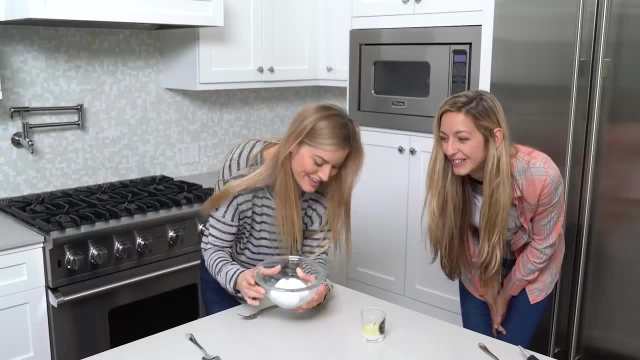 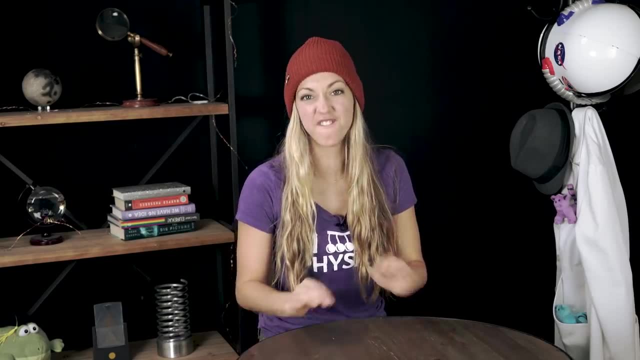 Just like that. That's so great, OK, Oh, it's awful. Justine was doing so well until I brought out my favorite piece of physics equipment, this metal bowl, Just kidding- The Van de Graaff generator. That's all. 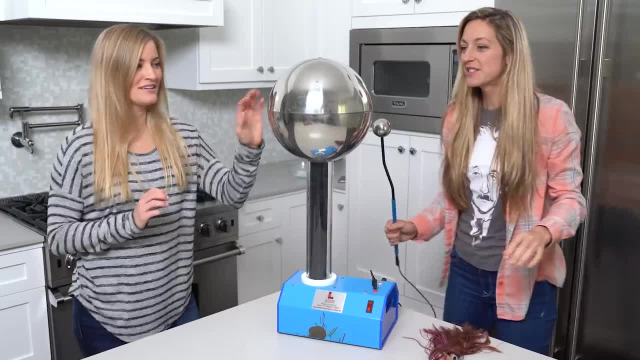 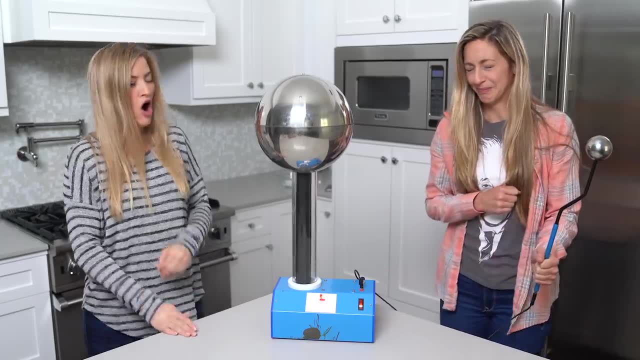 Whoa, whoa. OK, What Wait? I turn around and there's a time machine. This only produces 300,000 volts. I'm afraid to even touch it. OK, Oh, Oh, I'm feeling weird. You ready? 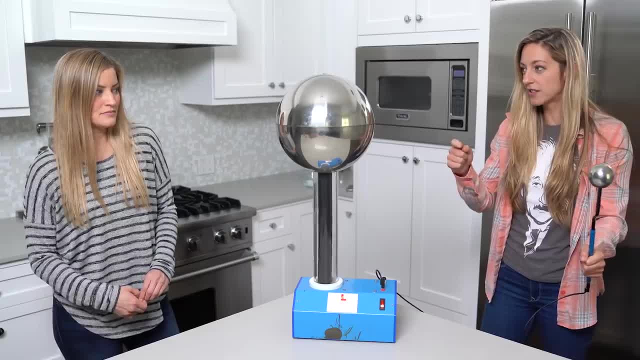 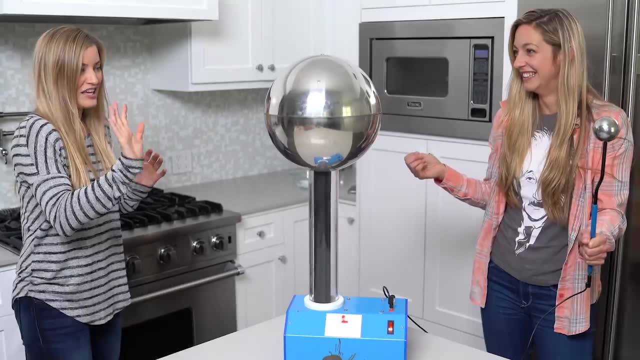 Yes, We haven't even started the video. Actually, like, if you use your knuckle, it's not so bad, Yeah, if you use your knuckle, Oh gosh, You can do it. Oh, I feel like I can feel. 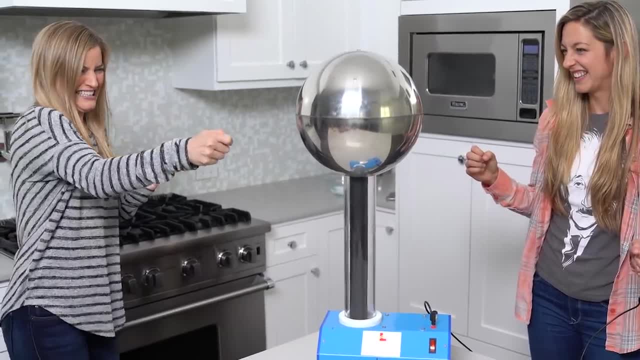 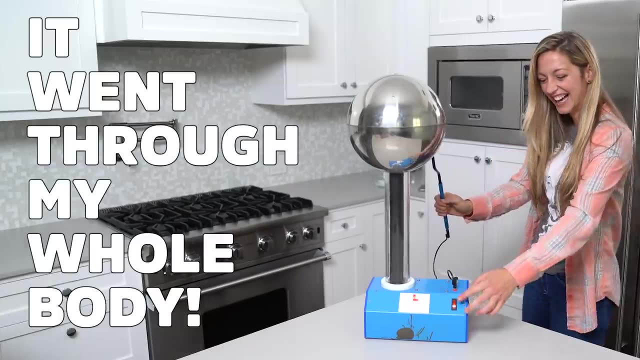 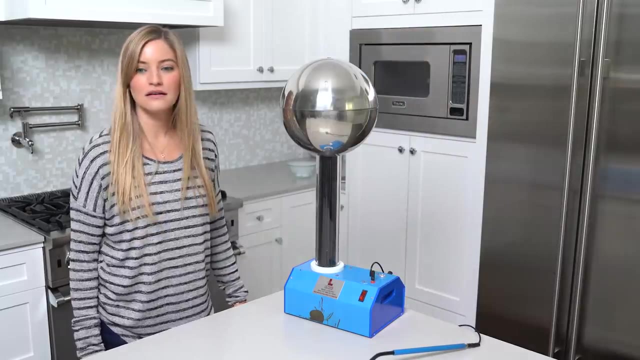 Oh my Yeah, It went through my whole body. OK, Scale of 1 to 10. Time, OK, The, it was like 45. I think I want you to maybe close your eyes. OK, What's happening? 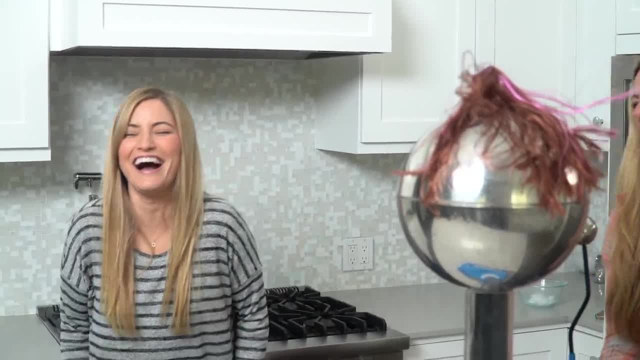 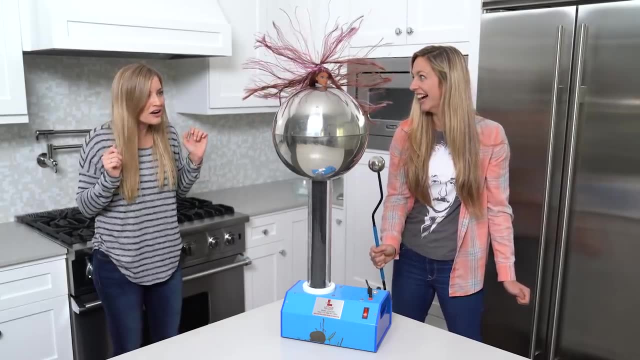 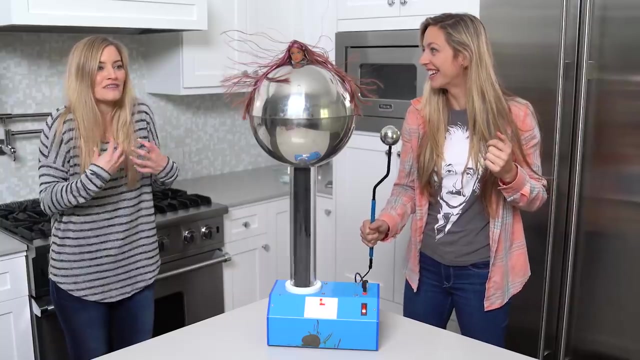 Open your eyes. That's incredible. Oh, Are you cooking to her? Oh, There we go. There's some good sparks. Oh my gosh, Did you feel that Like? I just feel it inside of my body. Yeah, 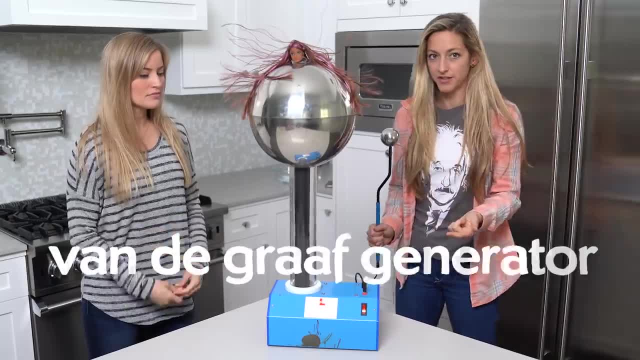 Like my jaw is tingling. I'm like: what is this? This is called a Van de Graaff generator On the outside of this metal sphere. it's such a high charge, It's like 350,000 volts. 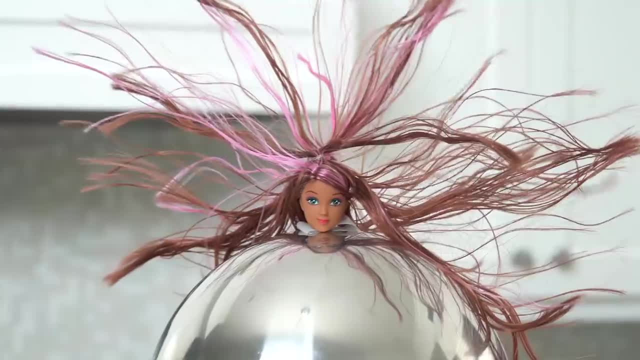 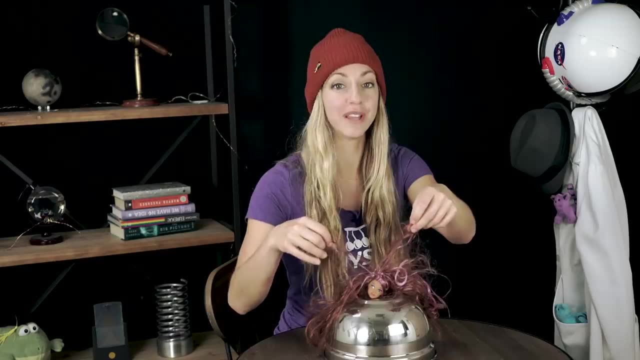 The generator causes static positive charges to build up on the doll's hair. but positive charges repel each other, So each one of the individual strands of hair wants to get further away from the other strands. so they stand up, They fly apart. 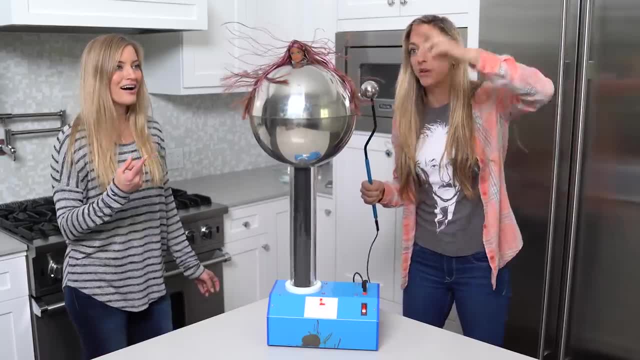 They want to get away from each other, essentially Like if I cut the hairs of this doll they would fly off. Some of these charges are coming off into the air and we're feeling them on ourselves. I'm feeling a lot of things right now. 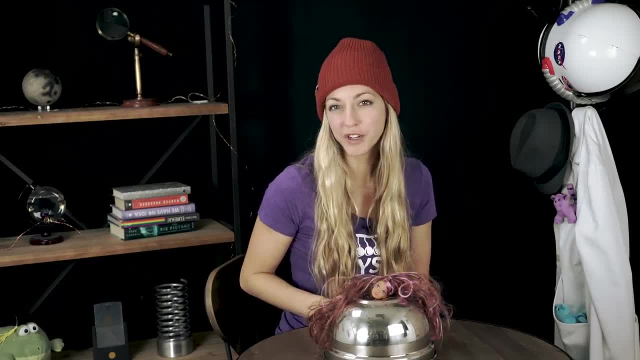 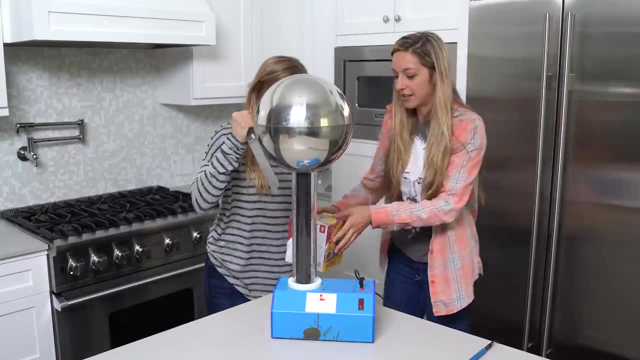 We tried to get our hair to stand up, but it may have been too humid for it to work. But what did work was Van de Graaff levitation. Wait, there's more, There's more. I thought we were done. Can you give us a little demo of the pro unboxing? 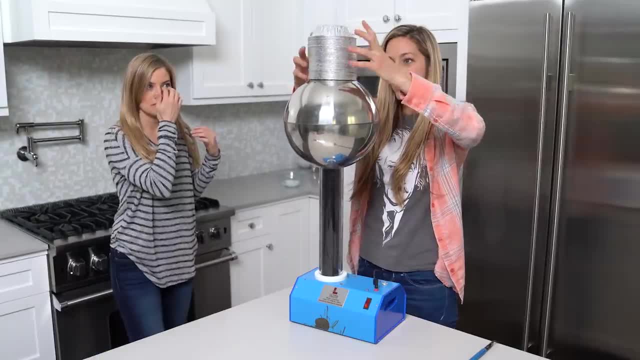 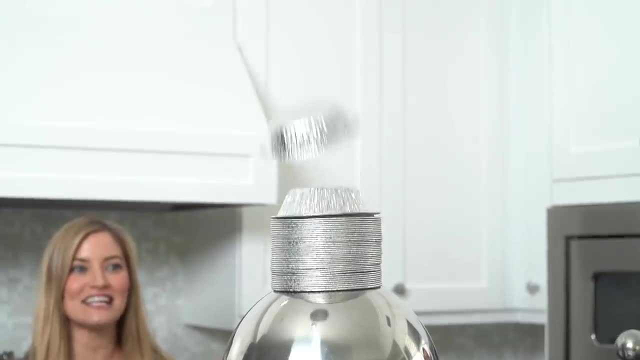 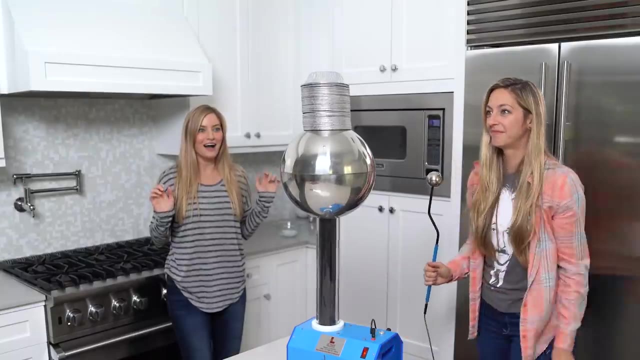 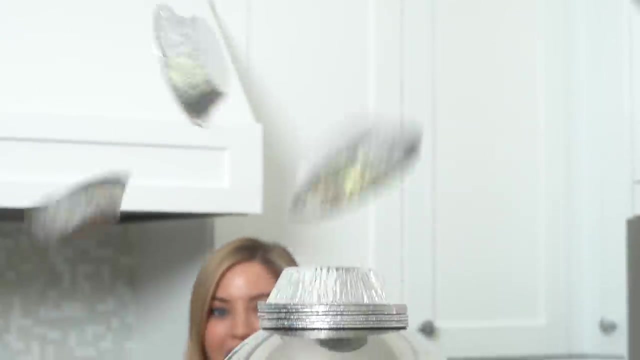 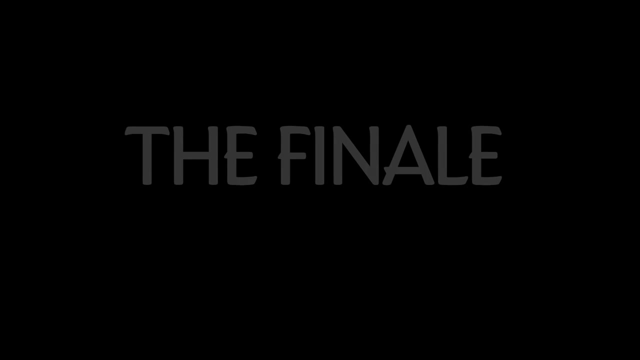 Oh, These are pie tins Here. It's kind of like baking with electricity. Yes, All right, No way. This is really incredible. This is so great. Yes, Yes, That was epic. It was beautiful, All right. 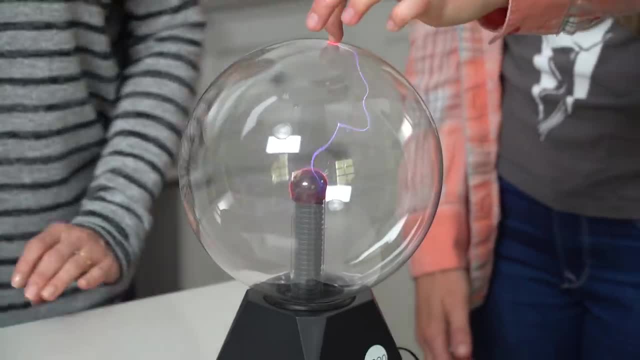 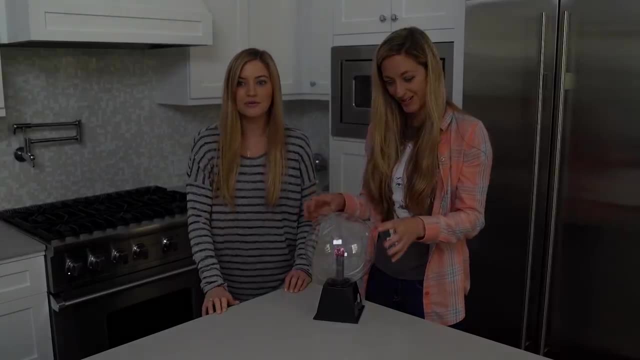 This one's not that shocking, I do promise. I promise I've lost all of my faith in you. now The finale: in my quest to scare Justine involved a plasma ball, Oh yeah. And this doll, oh yeah. 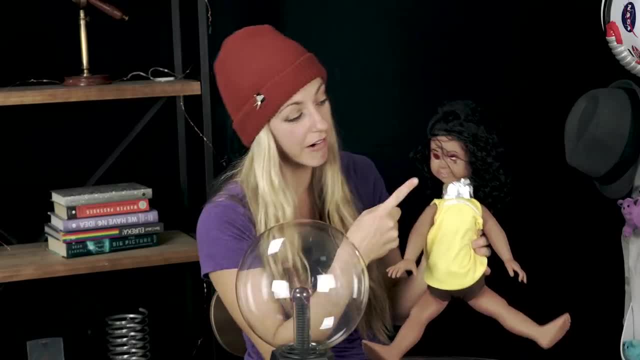 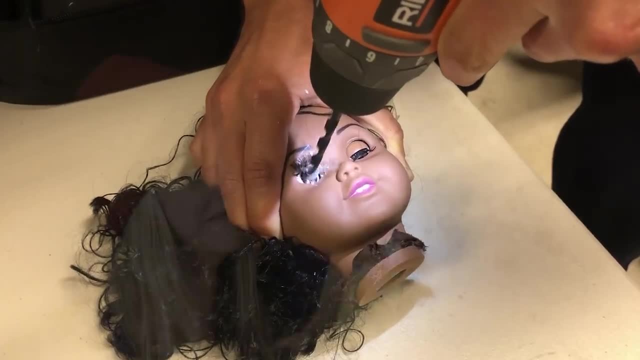 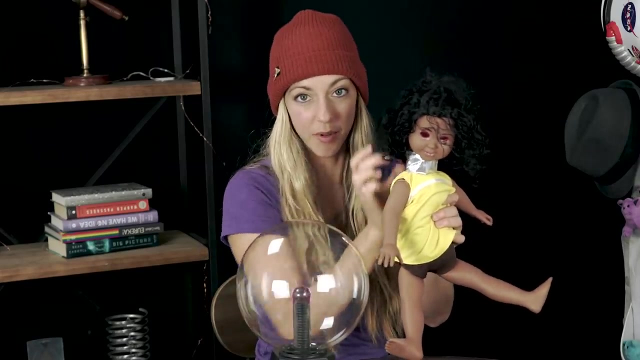 This is my creation- Creepiest thing I've ever seen. So I gouged out her eyes And I put some red tape over them And then I cut off her head And I- this is not normal- And I stuck a fluorescent light bulb up inside of her head. 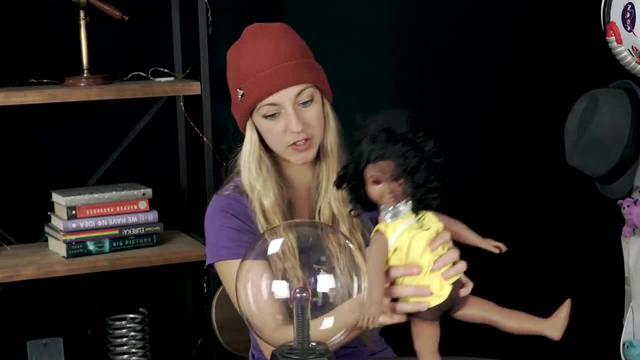 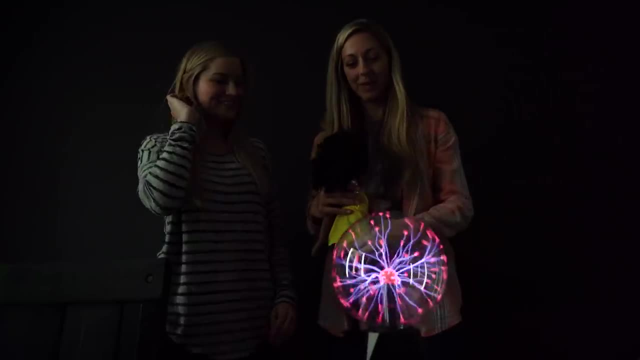 so that when you bring the tube near the plasma ball, it'll cause the isolates It'll light up. This is the weirdest one, All right, So I've got this doll that I brought you. I'm just going to bring it close to. 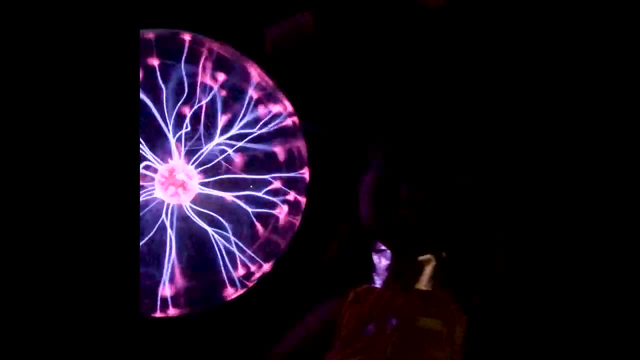 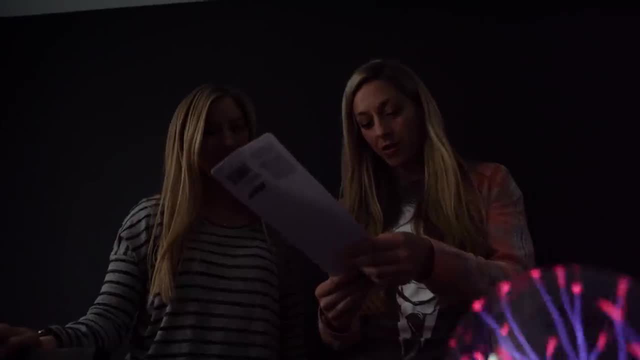 Oh my, What is this? That is super creepy. What have you done? Creepiness factor? This is probably your creepiest. This is just like a normal fluorescent light bulb. Whoa No, that's cool Yeah. 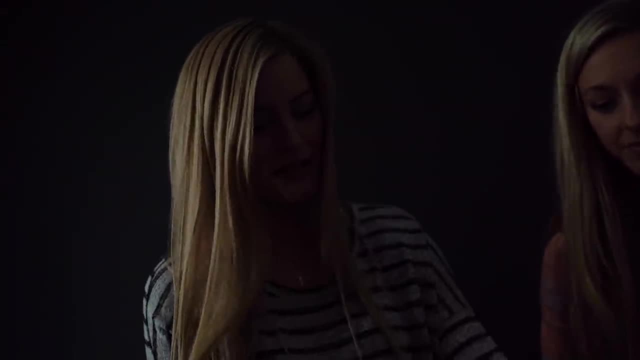 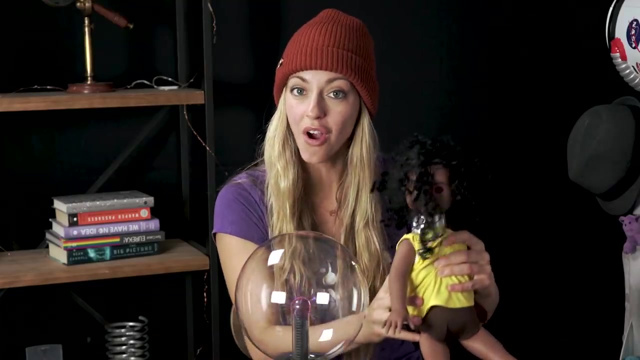 Isn't that cool, That's crazy, Yeah. So how is this happening? So let me repeat: The light bulb in the doll's head is not connected to anything. It's just inside the doll And it turns on when we place the doll near the plasma ball. 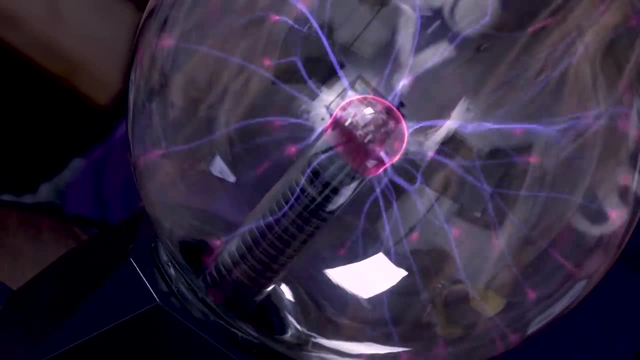 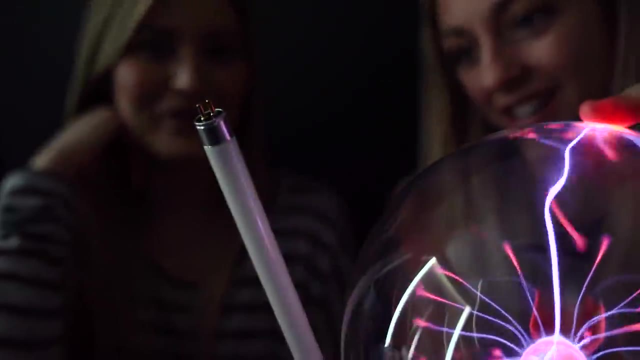 You don't even have to be touching it. The way this all works is that the center of a plasma ball has a lot of electrical energy in the form of an alternating voltage, But some of the energy escapes and smacks into the gas inside the fluorescent light bulb. 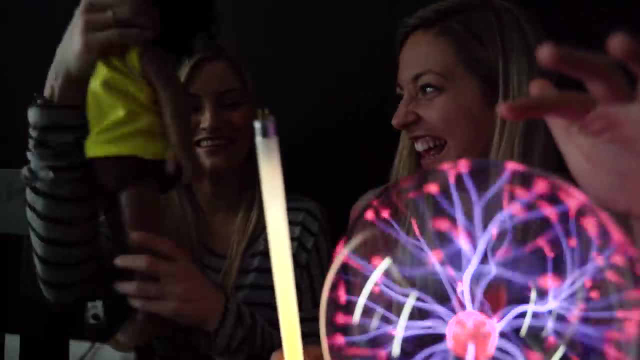 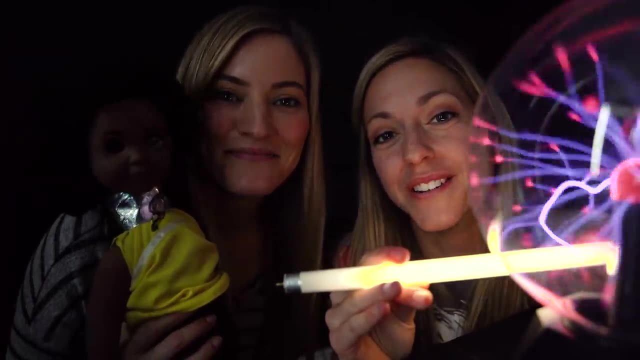 knocking off electrons from the atom in there and, in the process, emitting light. This is something I'll never forget. Who could forget? I wish that I could Thank you guys so much for watching this video. I mean the MVP right here. 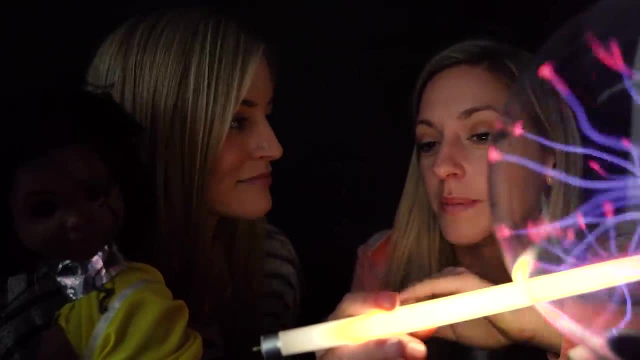 is Justine. It was just great to see her reactions to the creepy stuff, but also how cool you thought the science was. It was really fun. Yeah, thanks for bringing me into your world. Go check out the video on her channel. 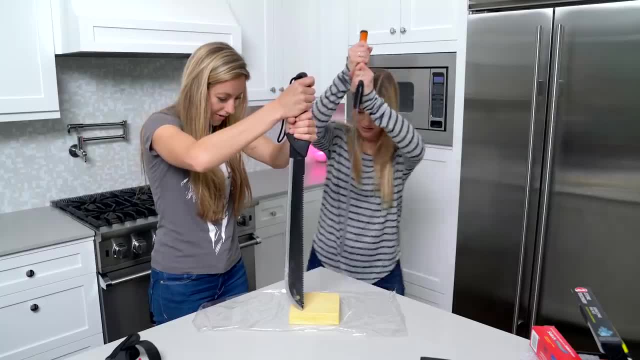 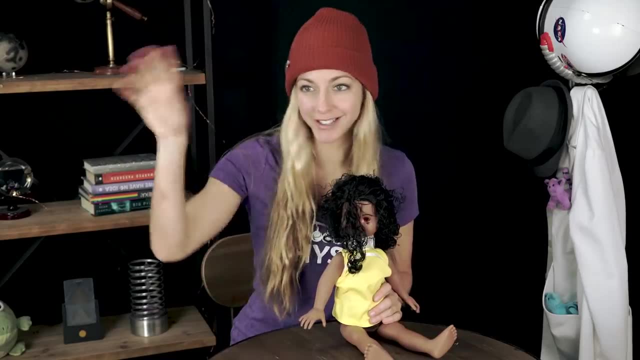 We made a video where we tried a bunch of kids' science kits that you can get off the internet, including digging for gems out of a plaster gem set. I'll link to Justine's video in the description and the end cards and so forth. 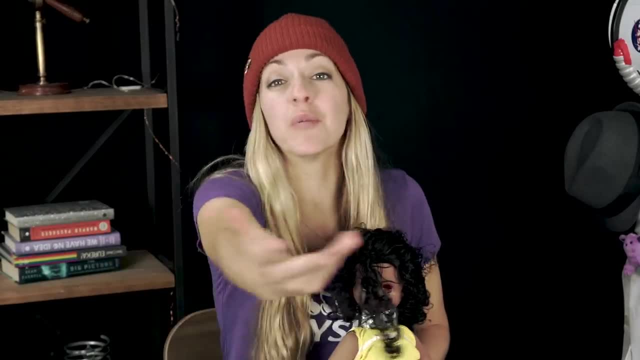 Let me know if you guys like this format where we have a guess on and we bring them into our world of physics, And if there's any guess, anyone specific you'd like to see on Physics Girl. Thanks so much for watching and happy physics. 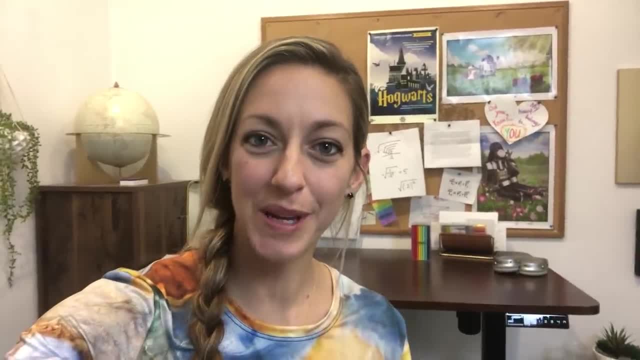 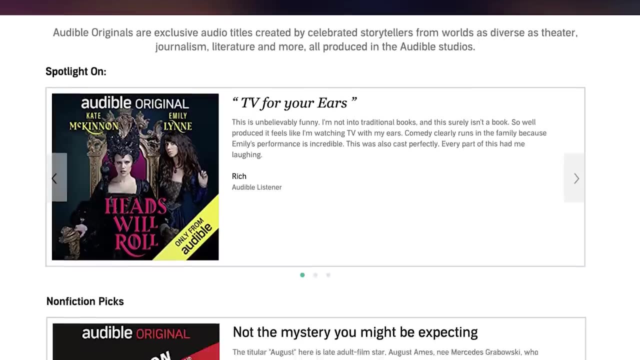 Oh no, Lost my microphone. I'd like to thank Audible for supporting PBS. Audible's collection of audiobooks includes Audible Originals- audio titles created by storytellers from around the literary world. For example, you could check out The Three Day Effect. 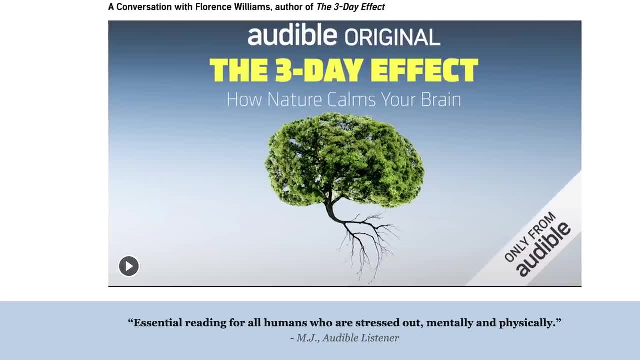 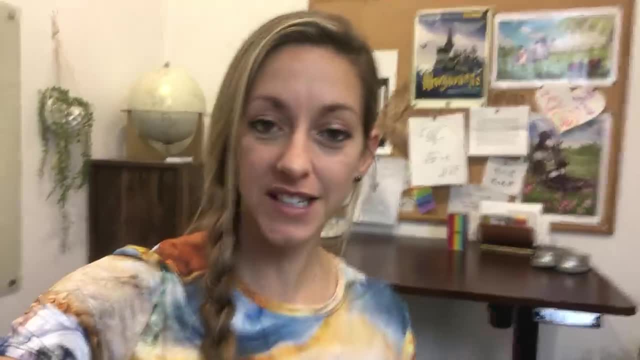 an audiobook all about how spending more time out in nature is better for your health and happiness. You could even listen to it while walking outside. For more information, go to audiblecom. slash physicsgirl or text physicsgirl to 500-500.. 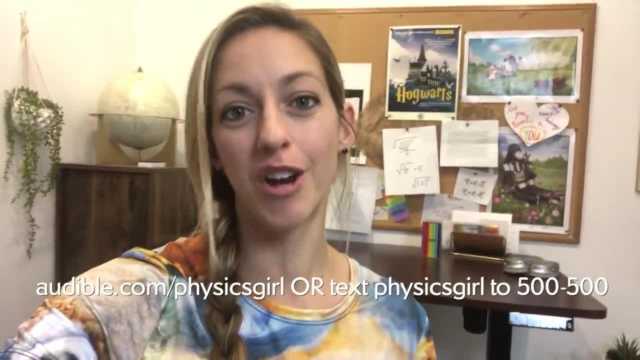 Members own their own books and can access them anytime. For more information go to audiblecom. slash physicsgirl or text physicsgirl to 500-500.. 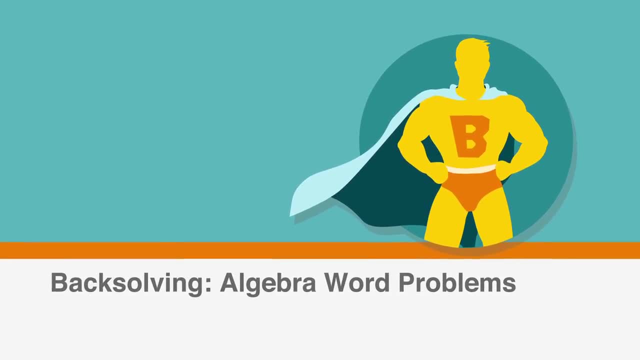 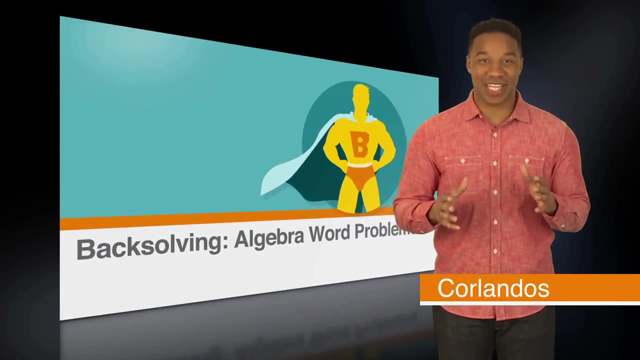 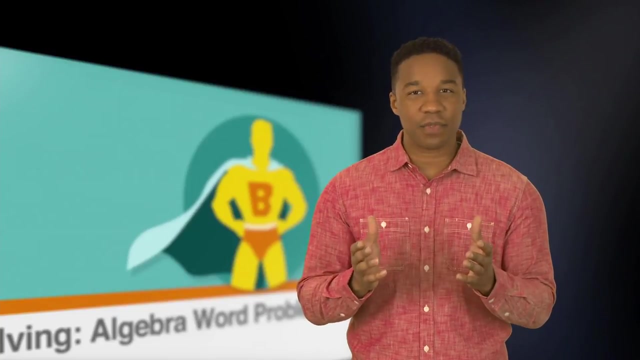 Back-solving is like your favorite shirt, You know the one that goes with almost everything. You can even use it with word problems, when you aren't given an equation. Anytime you're asked to find a specific variable, you can back-solve. Let's look at an example from